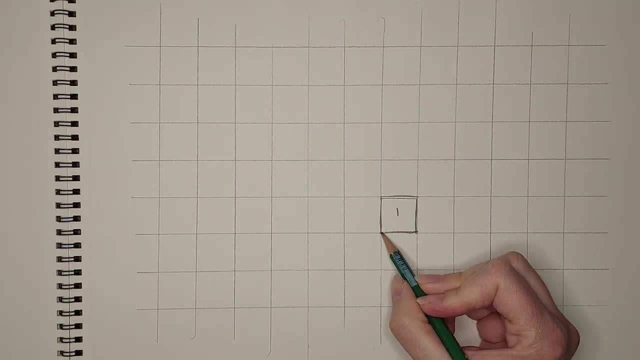 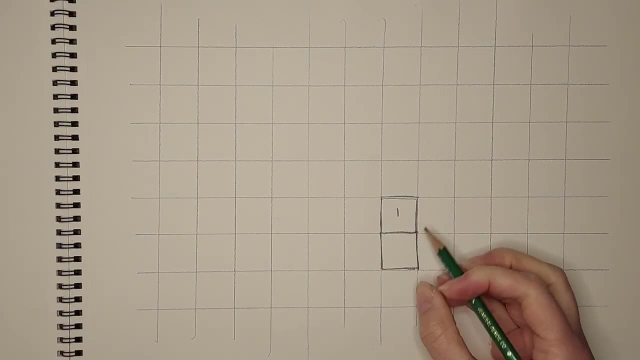 add zero to nothing plus one, So we're going to get another square of one. Now, if you don't, this doesn't make sense yet that's okay, just hang on. Okay, so one and one. Now, what we're going to do is we're going to spiral this spiral in this direction. So what we want to do is we. 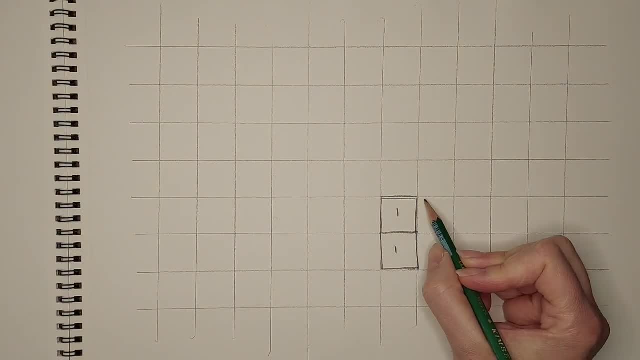 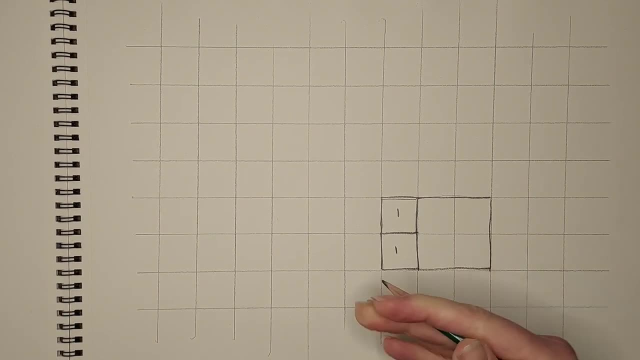 want to now say one and one. we're going to make another square. Everything is going to be squares in the beginning, And you're going to see that this, this sequence, is logarithmic. it gets big fast, but so we want to do one plus one is a square of two by two. 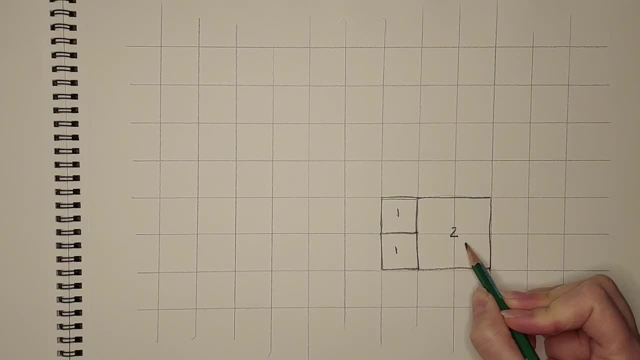 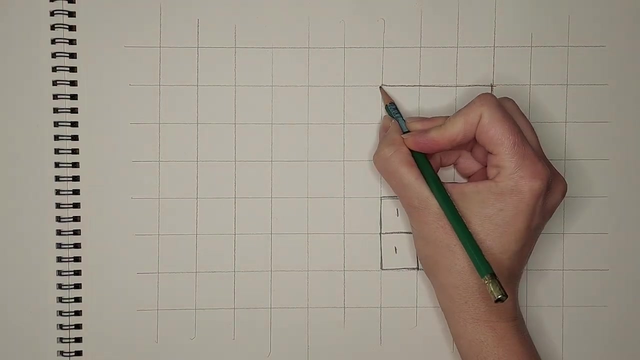 now, since we went this way and we're going out, the next one's going to be up here and we're going to add this line here which is three, one plus two. so we're going to go three and then up three and make a three by three square, and this is three. now our next square. 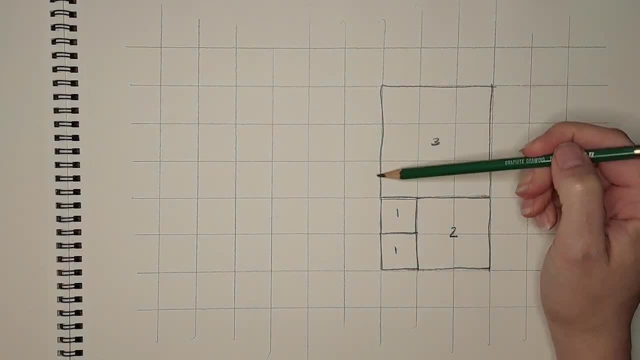 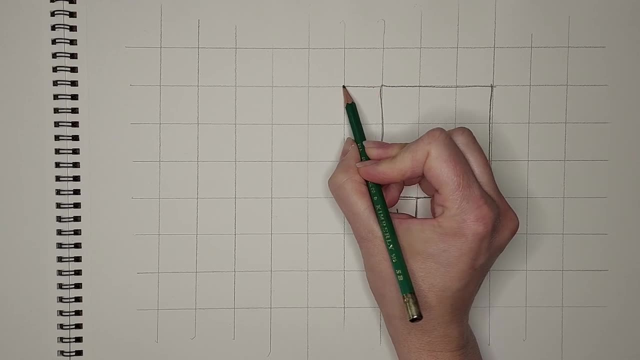 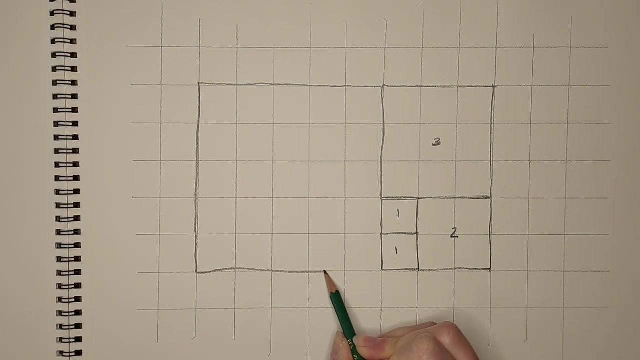 is going to be over here, and this is now going to be three plus the two, so it's going to be five. so three plus one plus one is another way to look at that. so one, two, three, four, five. down by five, over by five, we now have a five square. 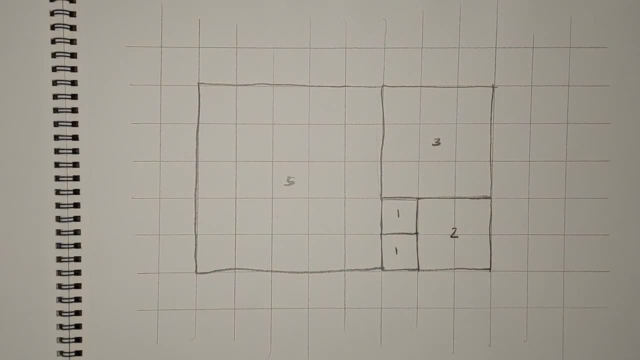 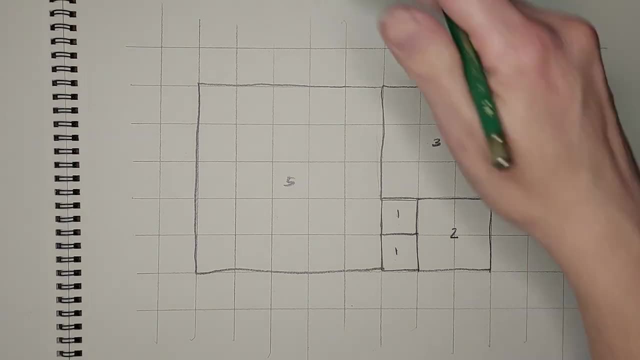 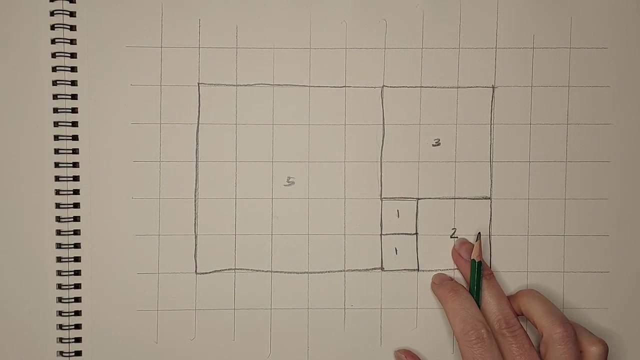 the next square would be here. going this way, it would be eight, then we'd have a 13 and it just 21, and it just keeps getting bigger. but i want to show you on this one real quick how you're going to do the spiral. so let me grab another color, okay. so now this next part. we're going to freehand a little bit. 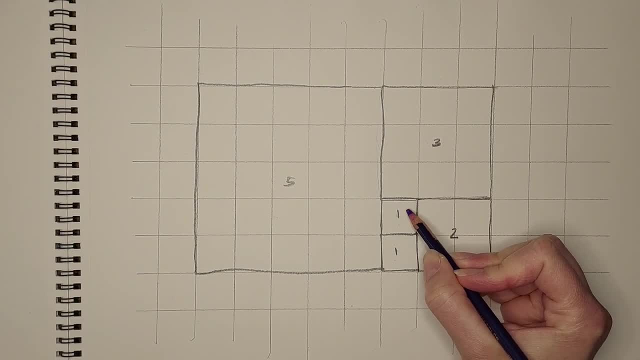 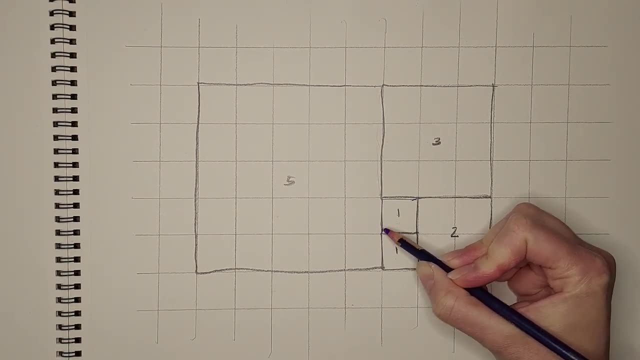 and what we're going to do is we are going to start in our first square and we are going to to start with this corner here and make our way to this corner here right, and you can just kind of sketch it in if you don't feel like you've got the curve right. just give yourself some time to. 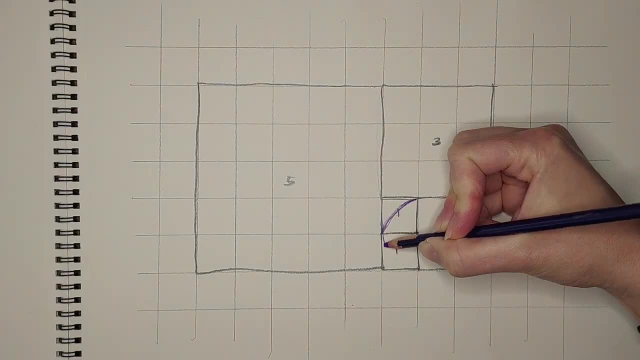 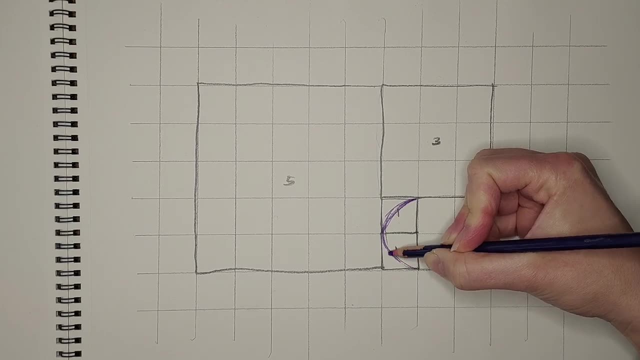 practice. so this one, now we're going to go to this one, and if you go like this, all of a sudden you can say like whoa, that's kind of a weird curve, and having that second one helps you know where you need to round it out a little bit more. now we're going to go from this one to this one, so